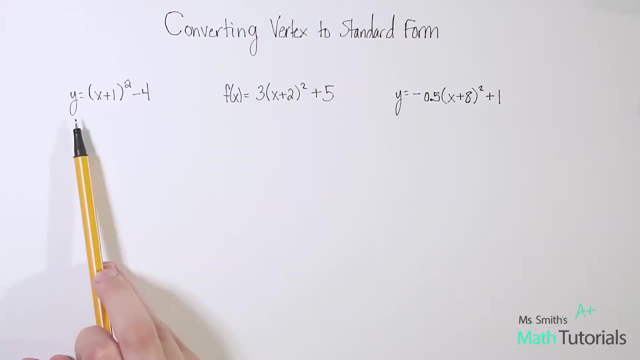 in vertex form. They are all quadratics, They're to the power of two, And I'm going to show you how to rearrange this into our standard form. And just as a little reminder, standard form is our: y equals n, Ax squared plus bx plus c. Okay, The first thing we would want to do is recognize that this is a. 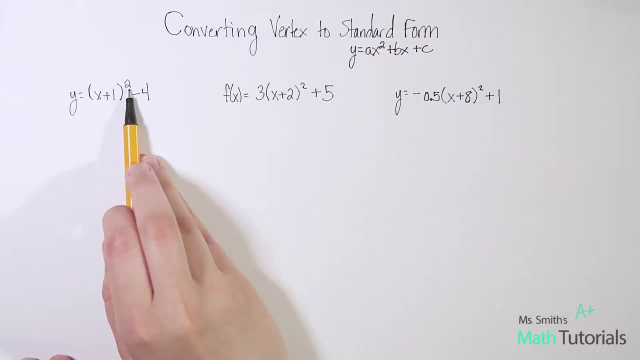 binomial squared, Okay, So we cannot. a lot of students want to try to distribute that power of two And they think, oh, power to power. exponent laws means that we multiply the powers. That doesn't work here, because this is a binomial That would only work for. 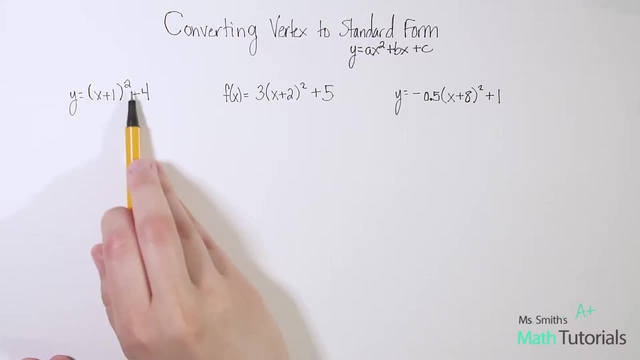 binomials. Okay, But since this is a binomial, I cannot distribute that, that power of two. But what I can do, and what this does mean, is that I rewrite it twice, So I put x plus one times x plus one. That's what this means. It's x plus one, squared, written twice, And then we have our minus. 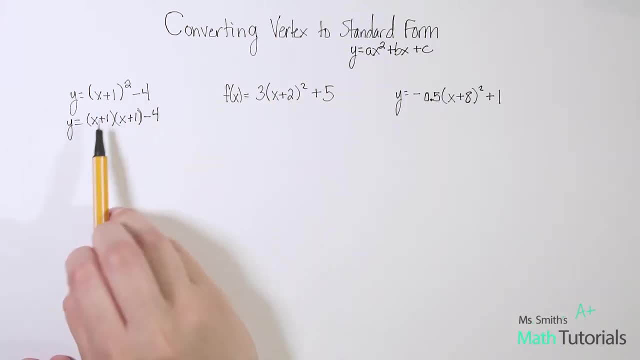 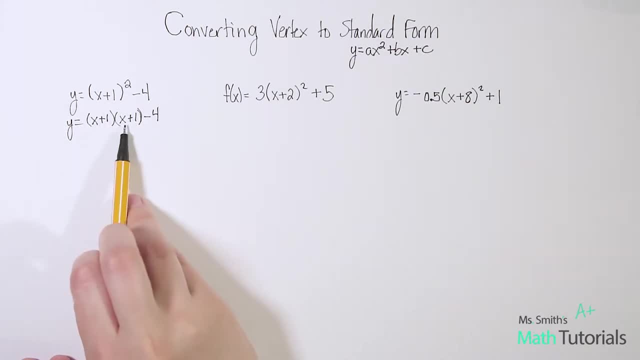 Times, a binomial, And hopefully you're thinking, oh, we FOIL those because we do. Okay, So we're going to FOIL these together And it's important we keep this negative four out here, this minus four, separate. Okay, So he's just going to kind of tag along as we go, but we're not going to use. 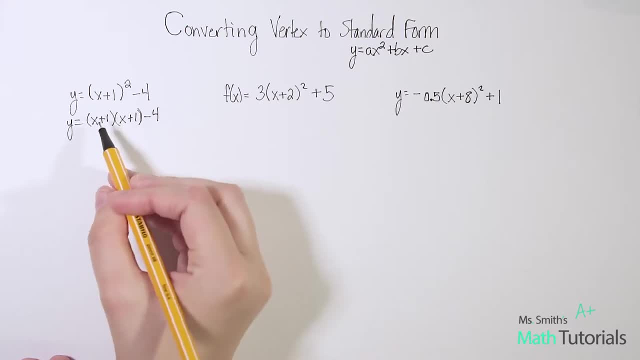 him until the very end. That'll be the last thing that we do, So let's worry about FOILing this first. So I've got my remember. FOIL the F means first. So this is: let's go ahead and rewrite it. 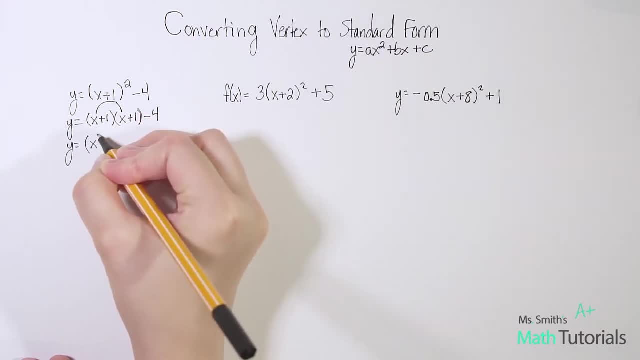 X times X, which is X squared. I'm using parentheses so that we can really see it'll be separate from this negative four. And then X times X is X squared. So our outer X went to the wrong place. Sorry, right here That didn't confuse anyone. X times one. 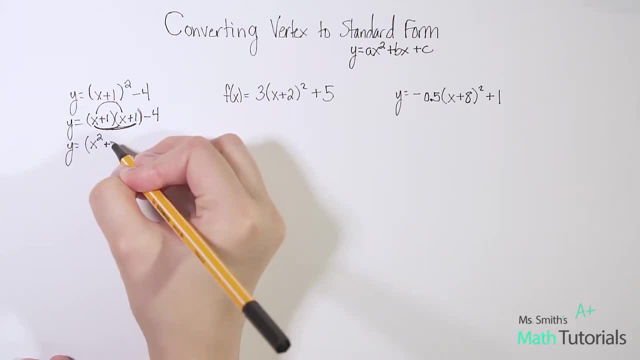 that'll be our outer, which will just be: one X positive, one X or just X. Now we'll do our inner right here: One times X is positive, one X or just X. And now our last one times one is just one. 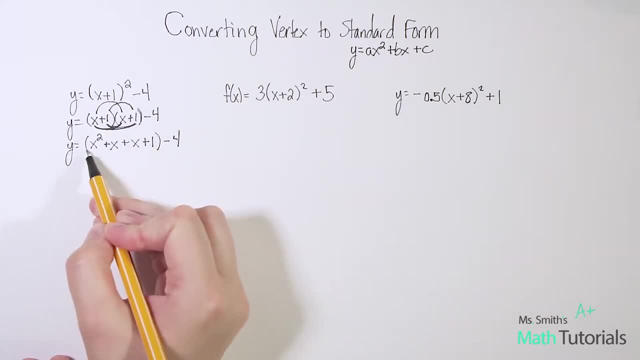 Okay, So now I have to understand that technically out here in front of these parentheses, is a positive one. There's nothing there, So that means there's an understood positive one. So when there's a positive one, there's a positive one. So when there's a positive one. 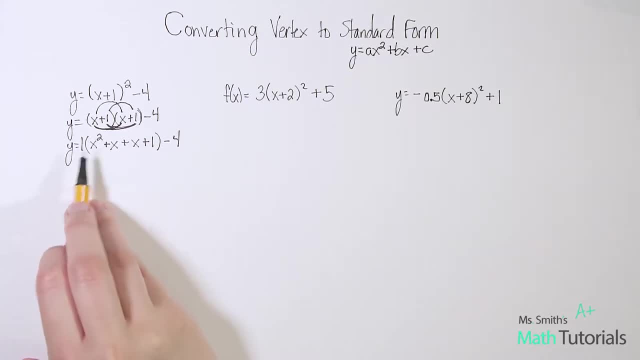 here. I technically need to distribute that positive one throughout the whole parentheses set Now because it's a positive one. we know it's not going to change anything right One times. anything is just exactly what you start with. But I want to show you this step because 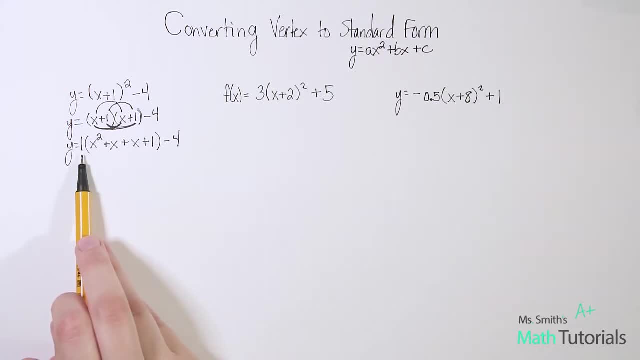 that number is not always going to be one. Okay, So in theory, here we are distributing the one one times anything, as we know, just itself, right? So I would just be left with X squared plus, and I can go ahead and combine these like terms. 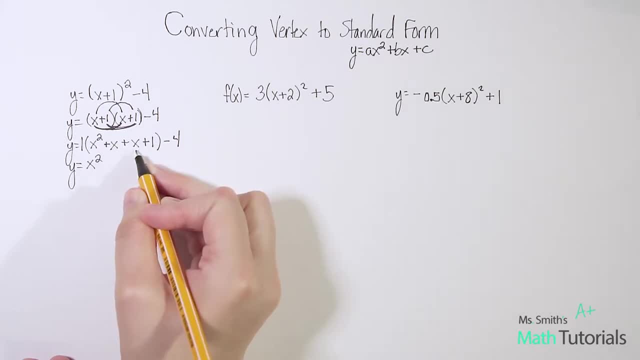 Just while I'm rewriting this, we know that X plus X is two, X, right. One plus one is two. So it's plus two X, And then positive one times positive one is just positive one, And then I have my minus four. So I finally, by distributing that one, the whole point of doing 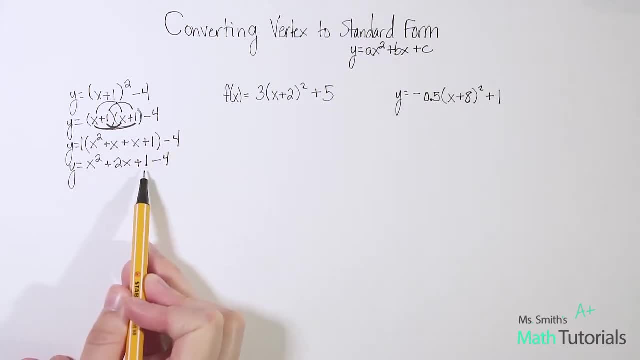 that was to get rid of the positive one. So I'm going to distribute that one and I'm going to the parentheses. So now, notice, my parentheses are gone. And now, as my final step, I can combine this negative four with this positive one. Okay, So we have Y equals. I got my X squared. 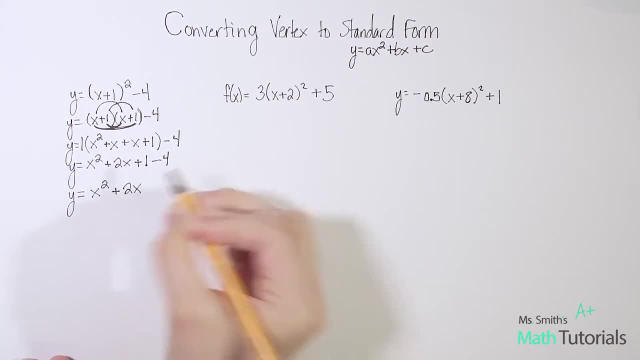 right, Two X plus two X And then one minus four. those are my like terms, just like these are my like terms here to combine that two X. these are my like terms here. So one minus four would be negative. three right, And I would check to make sure. are there any other like terms I can? 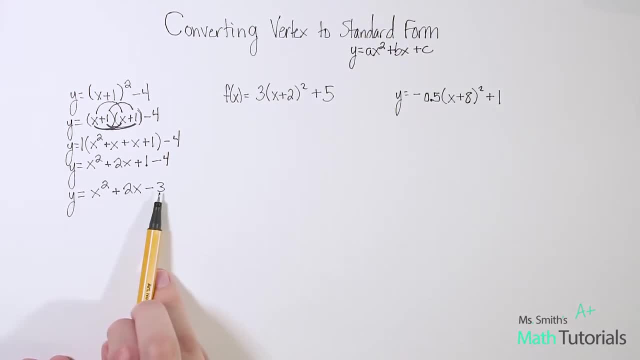 combine No, And then double check to make sure. am I in standard form? And as long as you've done this correctly, you should end up in standard form. but it's always good to double check, right, And so I am in that AX squared plus BX plus C form. Now what's cool about going from? 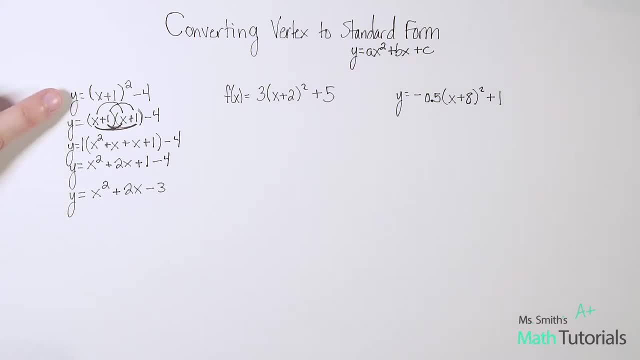 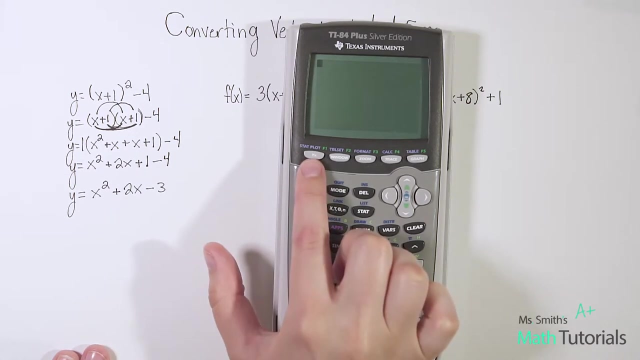 vertex form to standard form. so we've converted vertex to standard And what's cool about this is there's as long as you have a graphing calculator available to you, you can really easily check. Okay, So you want to bring your graphing calculator out and we want to go to the Y equals And the first equation. we're going. 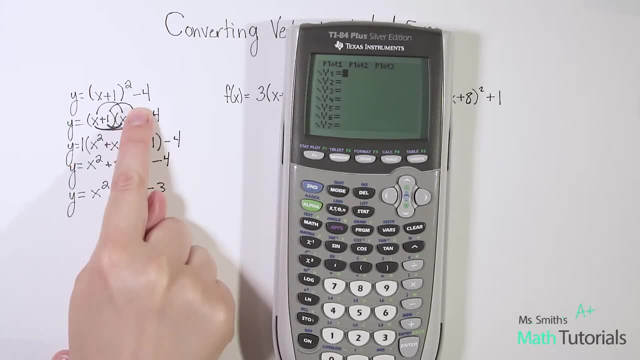 to type in is the original that they gave me in vertex form. So notice it's Y equals. Y equals parentheses X plus two X squared. And then I'm going to go to the Y equals, and the first equation we're going to type in is the original that they gave me in vertex form. So notice it's Y equals. 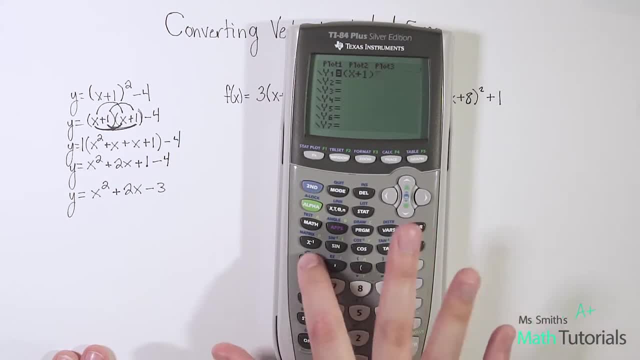 plus one squared, And then we have our minus four right. And then in my second line I'm going to type in: X squared plus two, X minus three. Okay, Now I want to graph these And if these are truly the same line, if I've done my work correctly, it should graph the exact same line. So I'm going to. 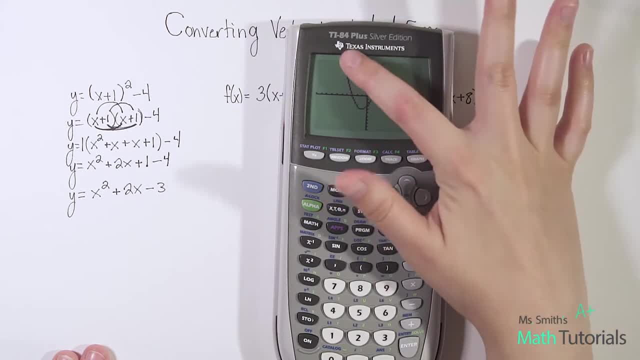 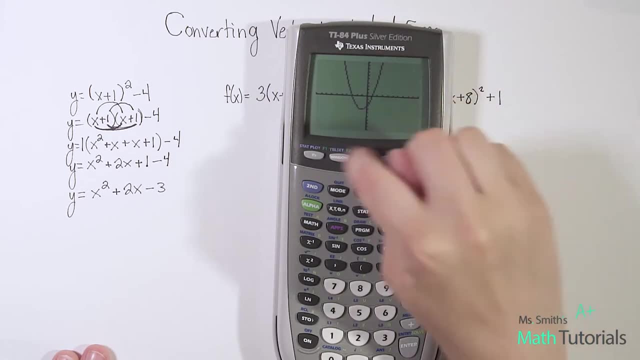 the exact same line. So you might say, well, it only did it once. Well, it's actually graphed, the two lines exactly overlaying each other. So the fact that I don't see anything else and I could zoom out just to make sure I could hit zoom three just to make sure there's nothing further out. 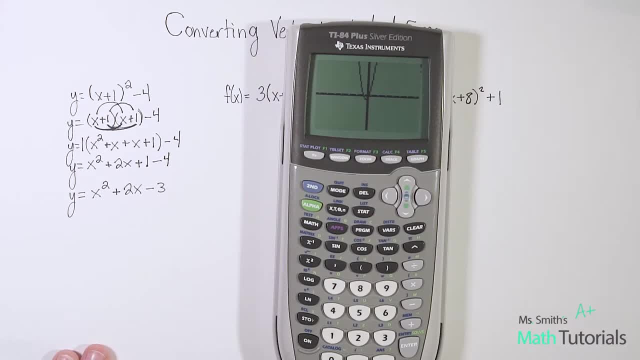 there. But, as you can see, it'll just be that one line, that one parabola, So I know I've done this correctly. That's a great way to see if maybe you've made a mistake along the way. So I'm going. 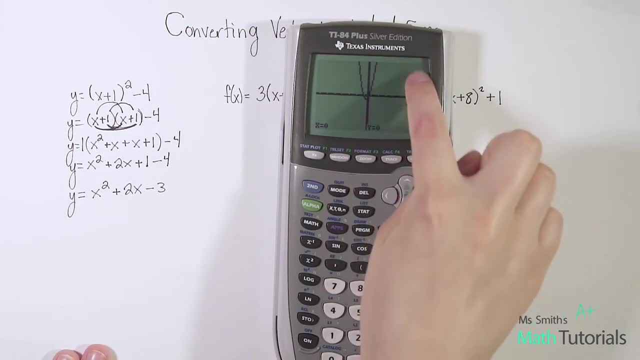 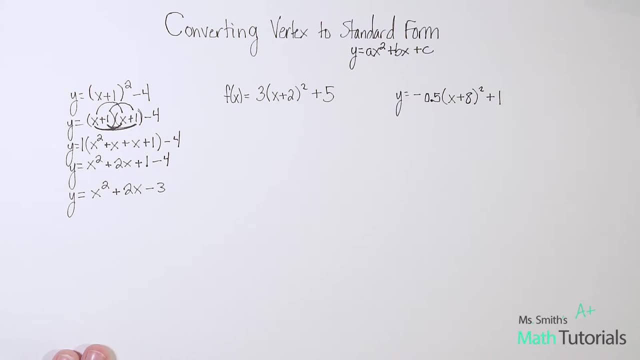 to do that And if you've made a mistake along the way is if you get two separate lines there, then you know two separate parabolas there, then you know you've done something wrong. So great little check you can use. Let's try another example. So for this one we have F of X equals. 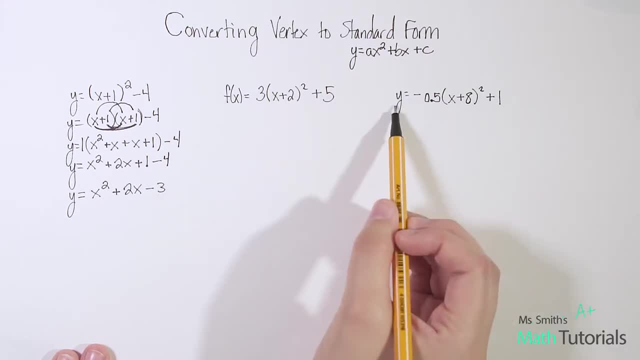 remember that's just the same thing as Y equals. Okay, I'd like to change it up so that you'll get used to seeing that F of X, So three times X plus two, squared plus five. So the real difference problem- and this problem besides the numbers being different, is the a value out front. so here it was. 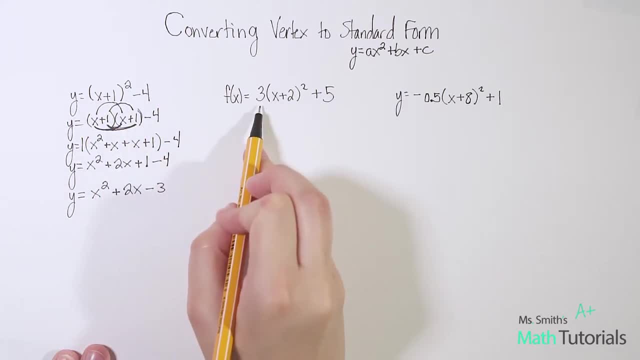 just a one, we didn't see anything. but here we have an, a value of three. okay, so that's going to just add on to our steps a little bit. just that when we distributed that one here. now we're going to be distributing a three when we get to that point. but it works very much the same. so we want to. 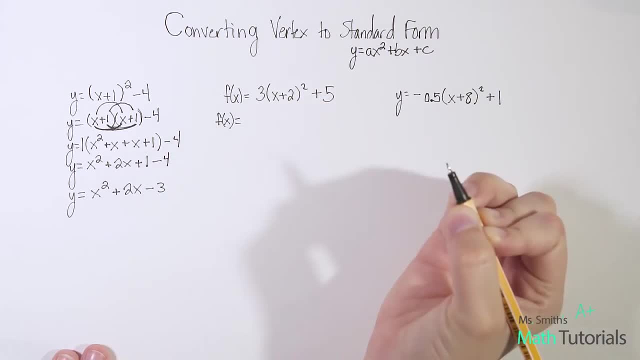 bring down our f of x or our y equals and the three I'm just going to leave out front for now. I'm not ready for him yet, but I do want to go ahead and recognize that x plus two squared is x plus two written twice right: x plus two times x plus two. and then I have that plus five hanging. 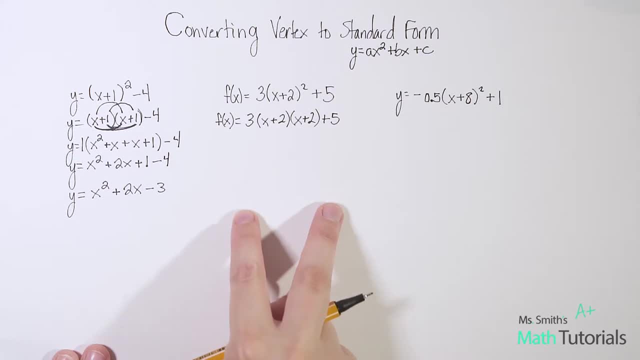 out. the three and the plus five are just going to kind of hang out until we're ready for them. the first thing I want to take care of is foiling you. okay, so I've got a binomial times- the binomial in the middle- here. I want to go ahead and foil them. 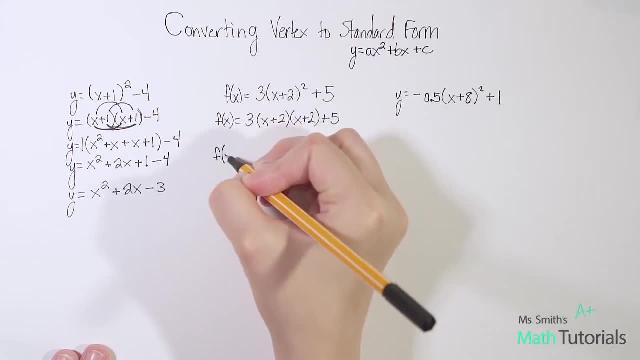 so remember, foiling is- and I'll go ahead and we'll start writing as we go. foiling is first right, so I'm going to use parentheses to show this is separate. until we're ready to take the parentheses away, x times x is x squared now our outer. x times two is plus two x. 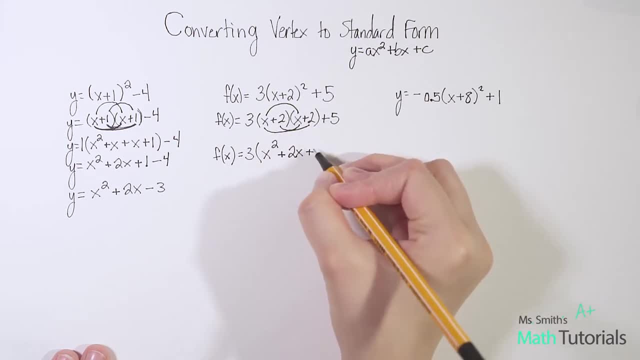 to squared twice. okay, so now we can just say x squared times four over two, x by two times x is plus 2x, and then our last 2 times 2 is plus 4, right, and then we have this plus 5 hanging out. now, of course, I do want to go ahead and combine those like terms in the center. 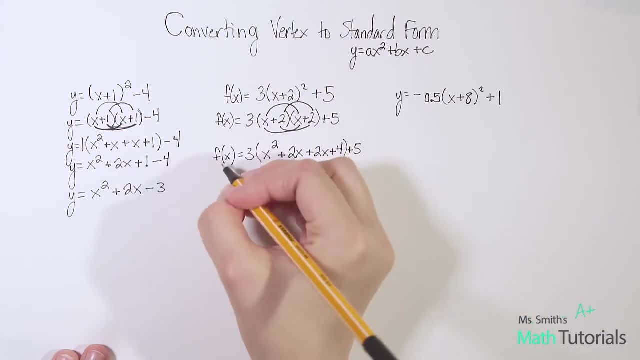 there and I can. i can go ahead and do that. I'm sure let's rewrite combining those like terms. so the zeroth of two plus x gives me 3 times x squared. now I'll get x squared plus 2.. that's gonna be 4x right plus 4, and then I have this little plus 5 hanging out on. 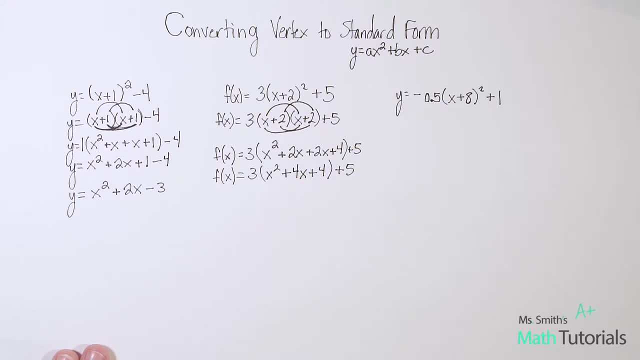 the outside. so probably the biggest student error that I see happens right here. students get this far usually and then they want to say, okay, 4 plus 5 is 9, but that's not what we actually do. first, remember our PEMDAS rules that if 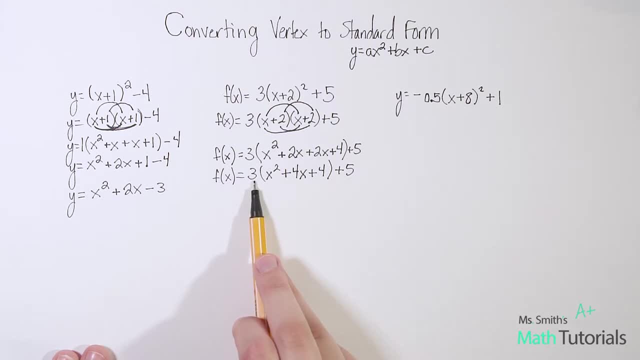 we've got something to multiply. so here we've got this 3 outside the parentheses. we have to distribute that 3 into the parentheses to make the parentheses go away. I can't just make the parentheses disappear and do: 4 plus 5 is 9. that's gonna completely change my answer. so remember that plus 5 or minus. 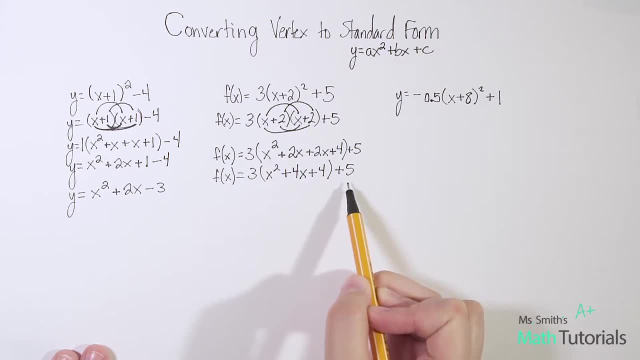 5, whatever it is at the tail end, you do that last. okay, we got to distribute first. that's why I really wanted to show that one over here distributing in, because we have to do that first officially. so let's do that again. let's go ahead. let's distribute that 3 in. so I've got f of x equals 3 times x. 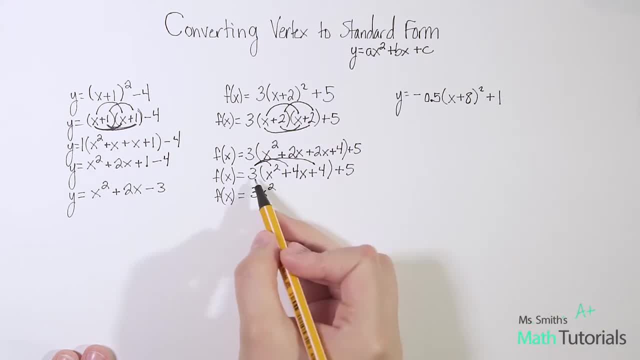 squared is 3x. squared 3 times 4x is plus 12x, and then 3 times 4 is plus 12. right, and now the parentheses have finally gone away. right, because I distributed the 3, so I can take that final step in. 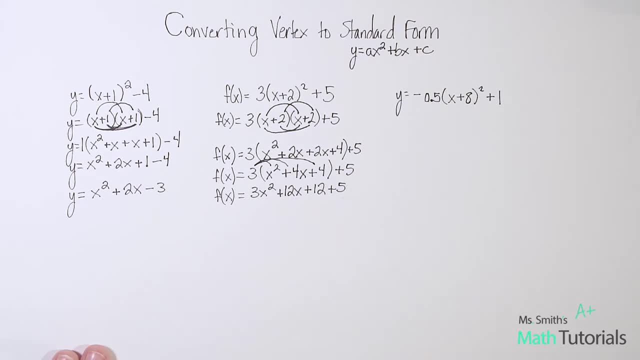 combining these like terms. finally, I can add that 5 in and that'll give me my final answer. so let's see: f of x equals 3x squared plus 12x, 12 plus 5, that's gonna give me positive 17. so you could see I went from vertex form to standard. 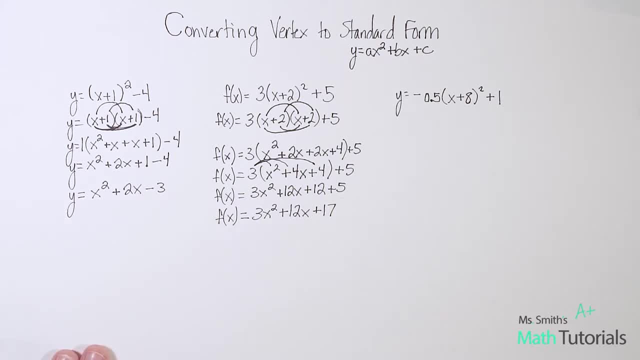 form alright? um, of course, I would always want to double check and say: am I in standard form, x squared x and c yes, and are there any other like terms to combine? no, okay, so i know i'm done. so let's look at one more example. so y equals negative 0.5 times x plus 8 squared plus. 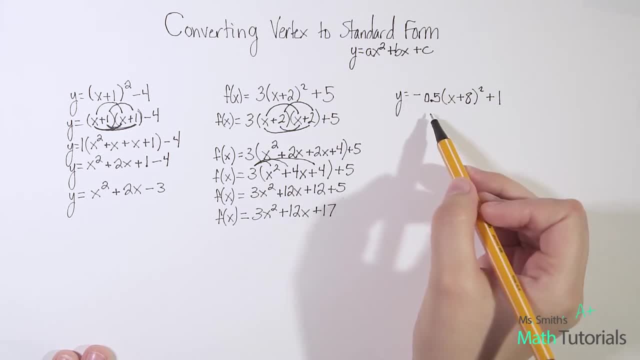 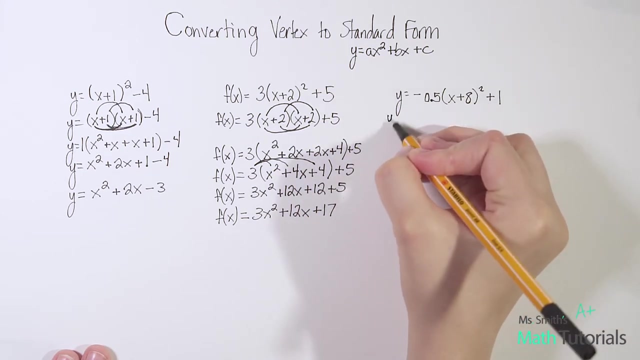 1. so don't be scared because there's a decimal here. sometimes they'll give you a fraction. don't let that scare you. okay, we solve it the exact same way. we just did those two, all right. first thing we'd want to recognize is we've got this x plus 8 squared, so we want to actually write it out twice. 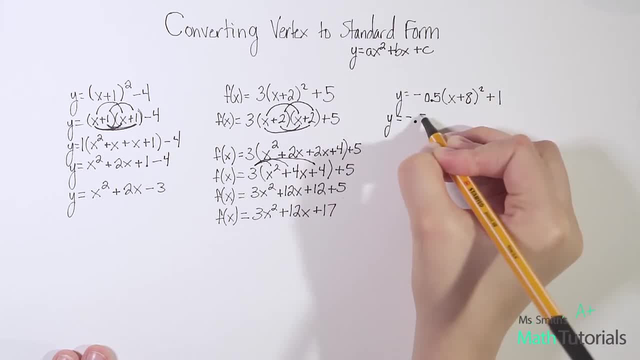 so y equals negative 0.5 or 0.5, same thing. and then we'll write this out: x plus 8 times x plus 8 and we have our plus 1 tagging along. remember the point: negative 0.5 and the plus 1 are just. 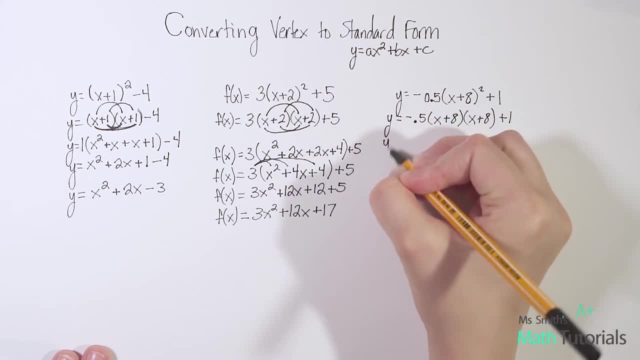 going to kind of tag along until we're ready for them. so y equals. let's go ahead and FOIL this: binomial times a binomial. so we've got negative 0.5 times all right, x times x, that's our first. is x squared x times 8 is positive 8, x, that's our outer, now our inner, x times 8 is plus. 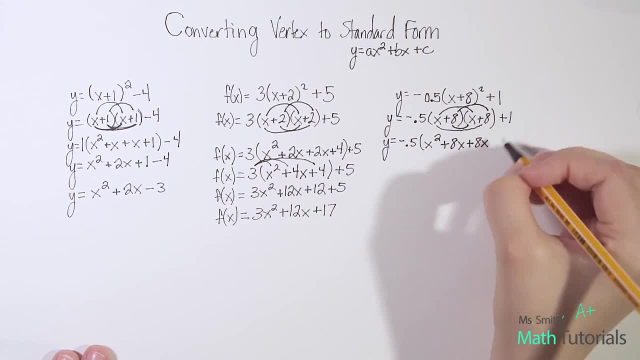 8 x and 8 times 8 is positive 64. okay, and then we have our end parentheses plus 1. so my next step: I don't want to just add 64 plus 1, I'm not ready for that yet. I've got a. we got this parentheses wall there that I've got to get rid of. I need. 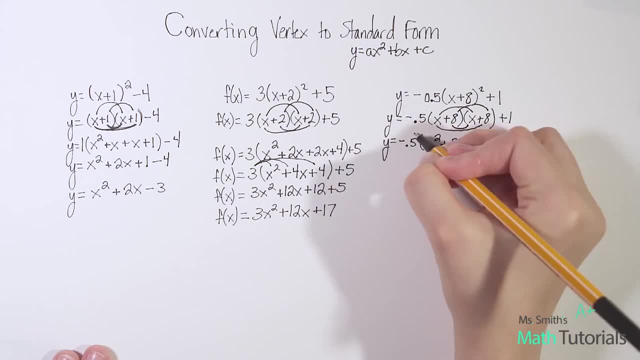 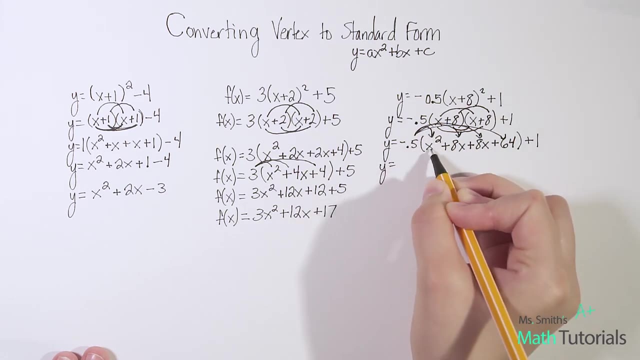 to distribute this negative 0.5 in first. okay, so we're going to distribute that to each part. so now we've got y equals negative, negative 0.5 times x squared. Well, that's just going to be negative 0.5 x squared right: Negative. 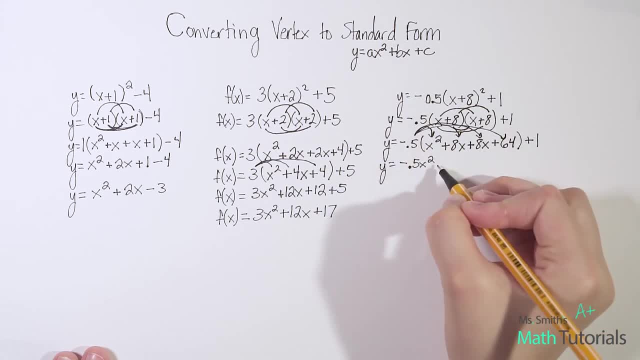 0.5 times 8x. Well, that would be negative 4,- sorry, negative 4x. And then if we went again- negative 0.5 times 8x- we'd get negative 4x, And then negative 0.5 times 64, that's going to give.